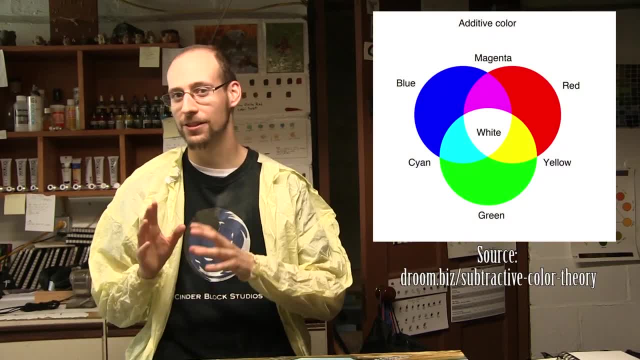 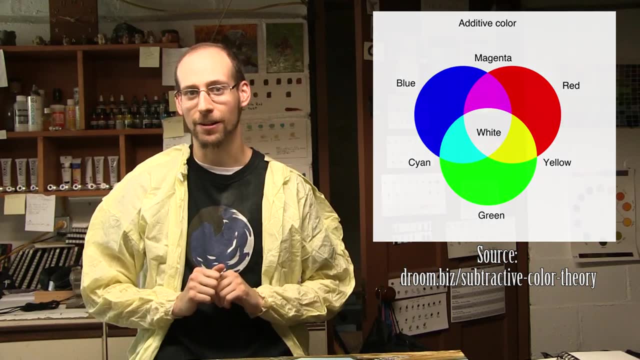 So you have color, So you have color, So you have color. So you have light: Red, blue and green, And when you mix these three colors of light together, you get white. The colors in the spectrum of light of red, blue and green are how our eyes perceive color. 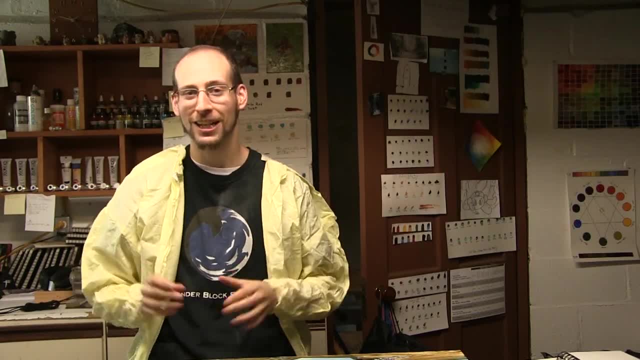 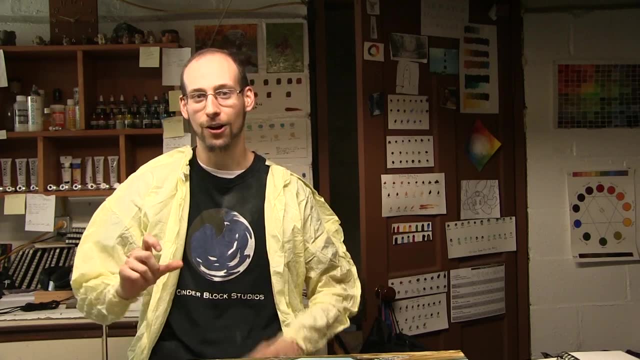 how light works in terms of spectral stuff in the universe, as well as how TVs and computer screens work. If you look close enough on a TV or you get a magnifying glass, what you'll see are those three indicating colors to create any variety of color you can imagine. 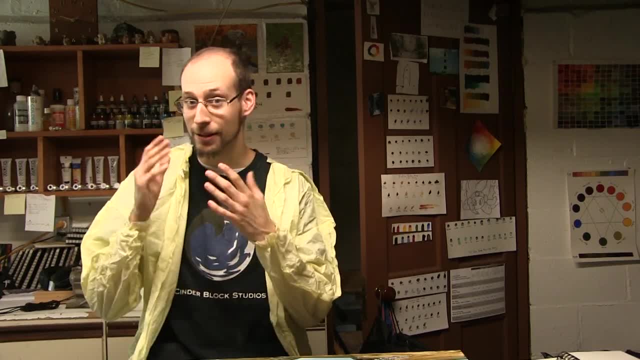 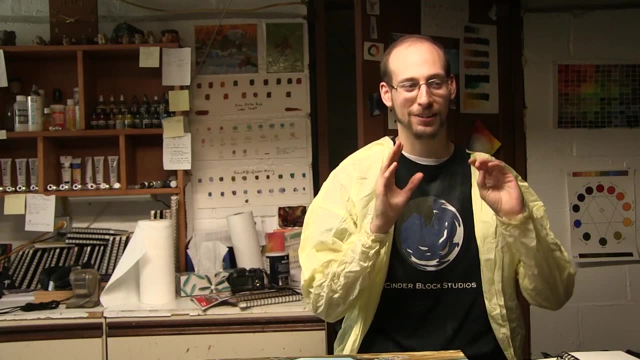 And, of course, when you mix the three colors together, you get white, and any color that's just darker or black is just the absence of that light. However, on a science standpoint, artists use a form of color theory known as subtractive color. 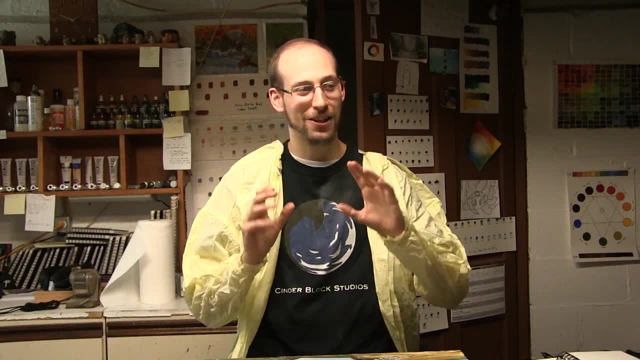 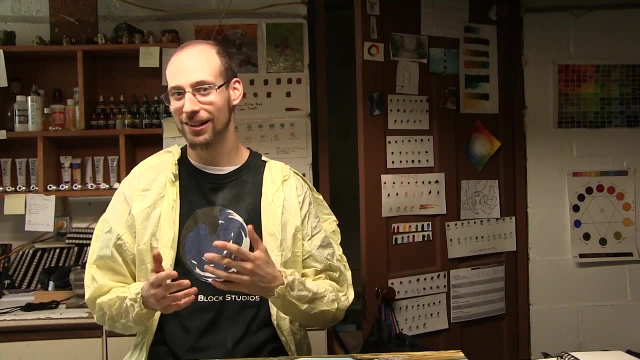 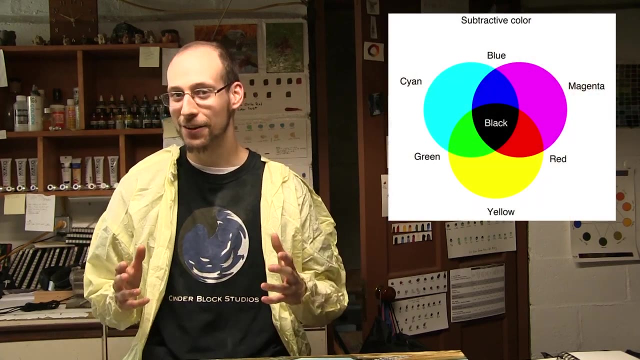 This is how pigments work. Pigments, unlike colors and wavelengths of light, absorb and reflect light to give us the color. And while the primaries share a similarity of red and blue, with additive color, rather than green, you get yellow. And when you add all three together, rather than getting 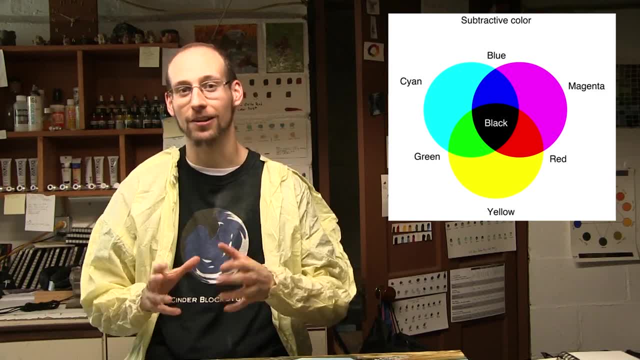 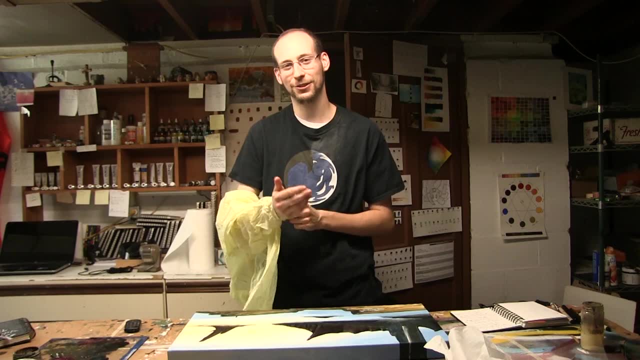 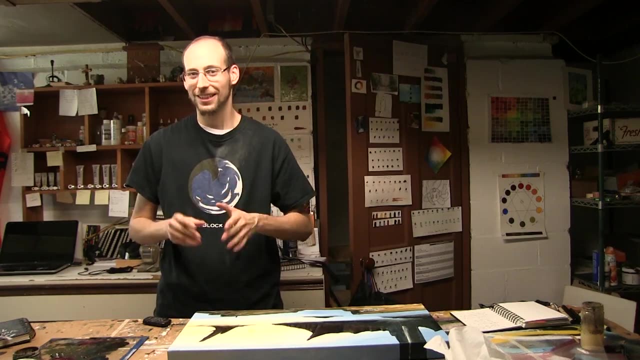 white, you get a brown color. But with all of this weird science-y stuff aside, we still have not answered our initial question: Are black and white colors In terms of art, in terms of pigments? yes, black and white are colors because they're pigments. 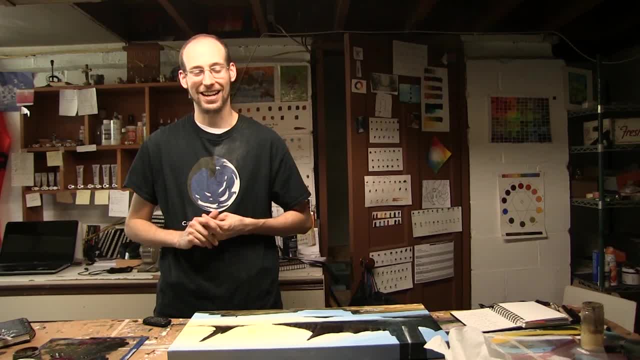 And yes, if you're a digital artist, you can actually play with additive color in a program like Photoshop and it's interesting and kind of weird to do that, but it's a great way to make your art look better. It's a bit of a disconnect. 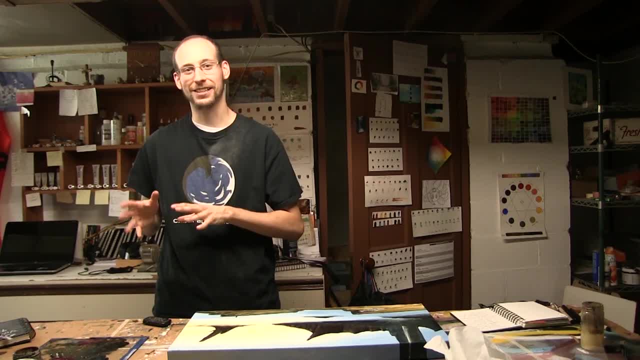 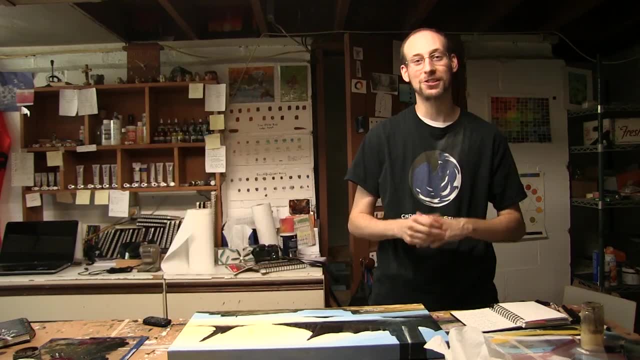 But the way the pigments behave in treating black and white like colors. that's how art works. That's how everything works in the real world, As long as you're not talking about the colors of light. Now, of course, a science buff will probably try and argue otherwise. 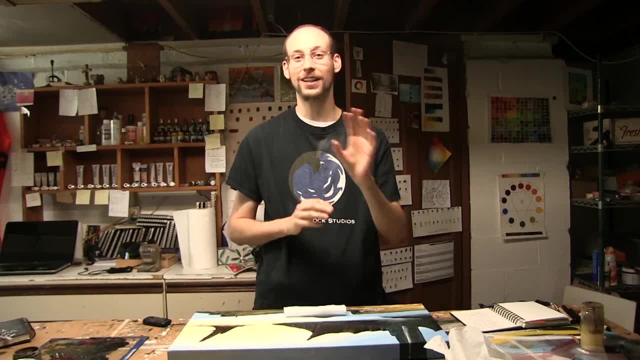 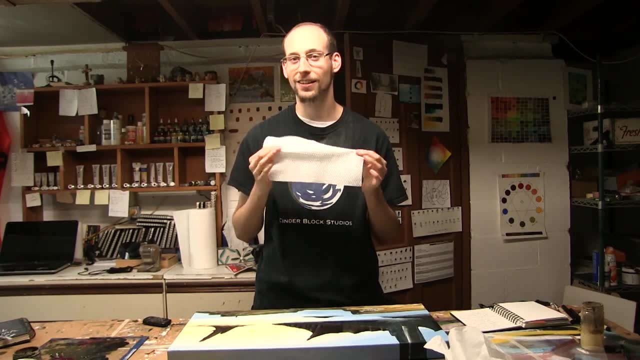 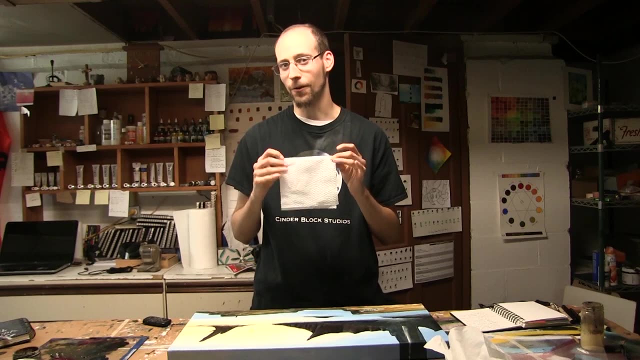 I highly anticipate several of them in comments. But despite all of the science-y guys out there, think about this as a simple example. This paper towel is white. It was probably dyed or bleached white to give it this color, This particular paper towel. if we were standing in the dark you couldn't see that it was white. 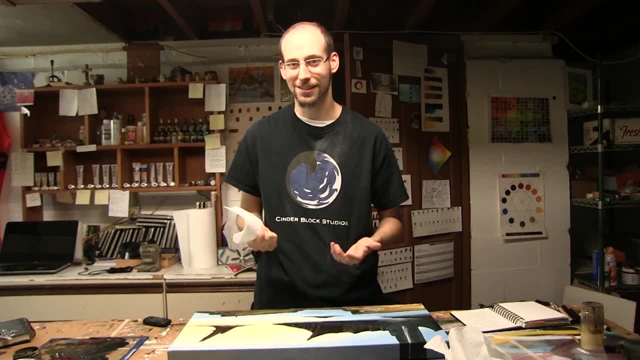 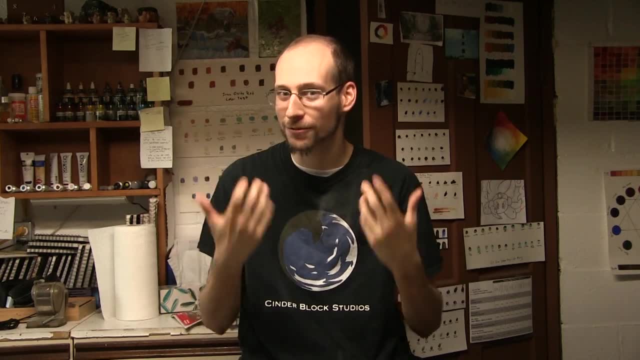 But that doesn't mean it's not white anymore. It's still white, whether or not you can see it. So, to review, black and white are, yes, they're tonal values in terms of light, But in terms of the art world, in terms of color theory for an artist, you have to treat 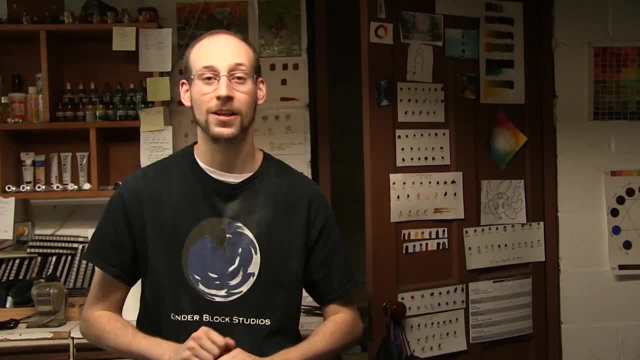 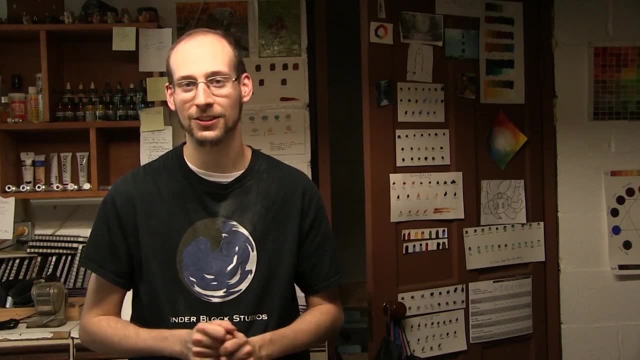 them as colors. If you don't, you're probably going to be messing yourself up. So the color theory behind subtractive color is really what every artist is taught from, whether they're day one, as a hobbyist or something. even that, I think most people 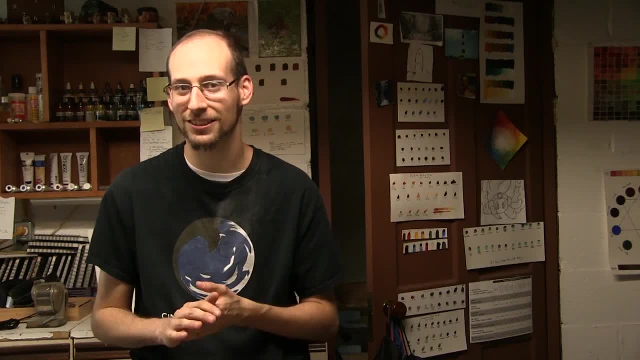 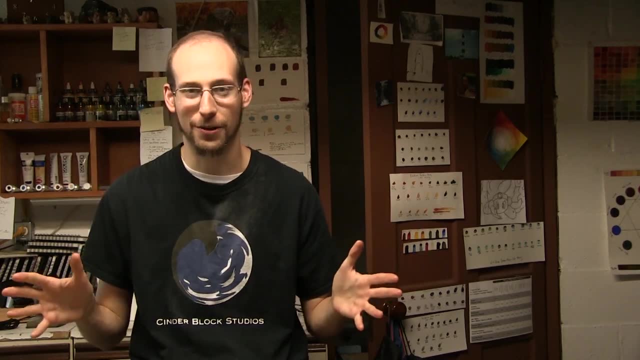 learn when they're a little kid. You get a little pan of watercolors or crayons. You mix yellow and blue and you're going to get green. You mix red and blue and you're going to get purple. You mix red and yellow and you're going to get orange. 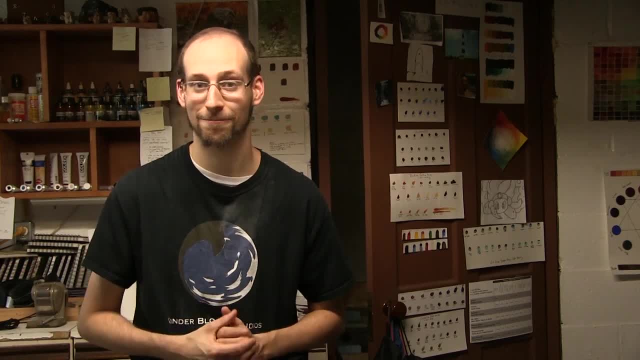 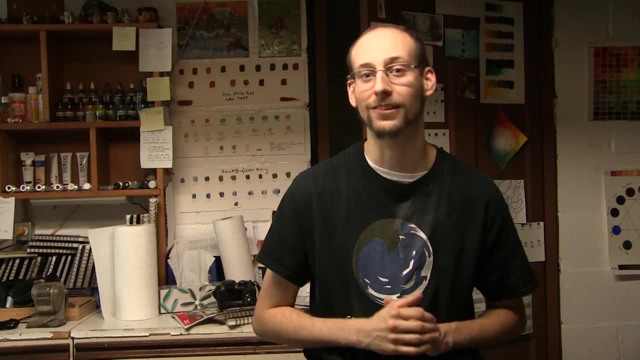 And if you mix all of them together, you're going to get something that resembles black. The one instance I do think is worth noting for a fine artist is if you're more or less going to be painting with light. There's something with. 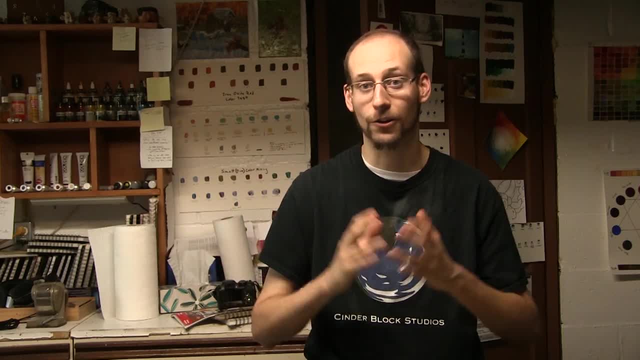 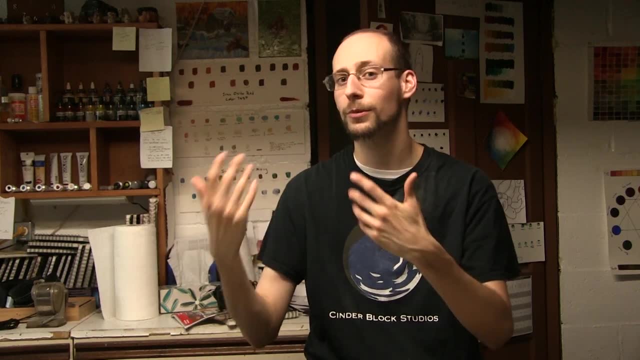 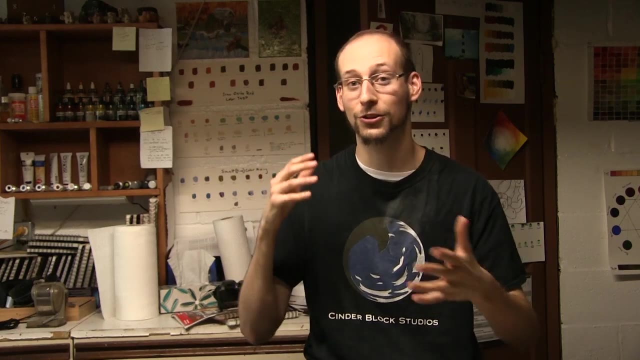 There's something with doing large-scale outdoor projects, things like large installation work, where perhaps you're not going to be painting an image on a wall but displaying an image on a wall or multiple images on a wall with light. When you do that, you have to understand the properties of light, because when you start, 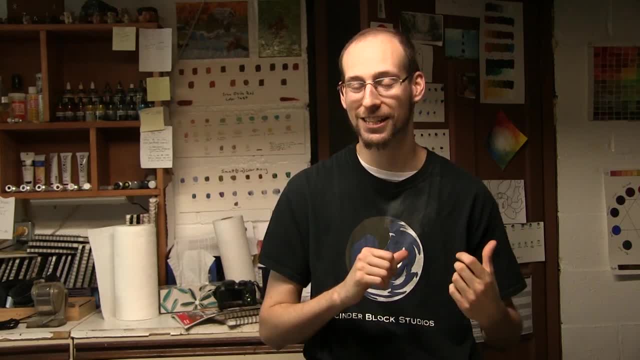 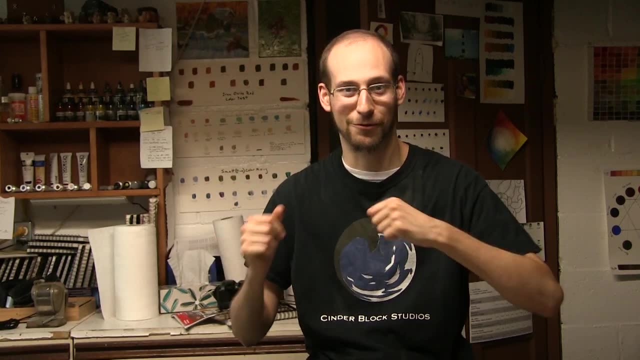 trying to mix colors based on the pigment subtractive way, and you're showing maybe a blue and a green. on a building like this, that's going to change the color because light works differently. So I hope you enjoyed yourself. I hope you enjoyed your science lesson for today and how it relates back to art and 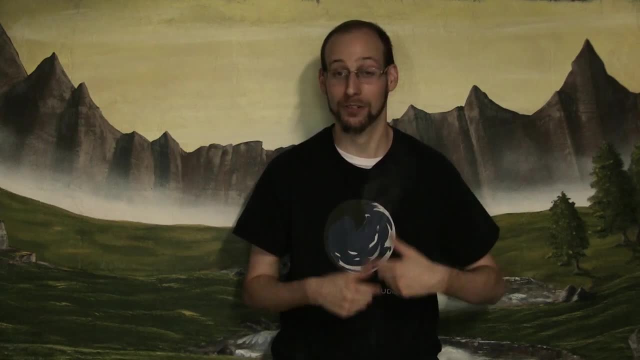 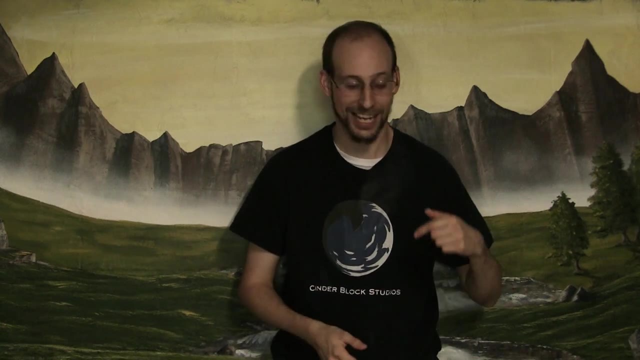 for color theory. Part of this video was inspired by me watching a recent episode of SciShow. It was about illustrators and artists that made a difference in the scientific community, And the guy that kind of pushed forward this idea of additive and subtractive color was 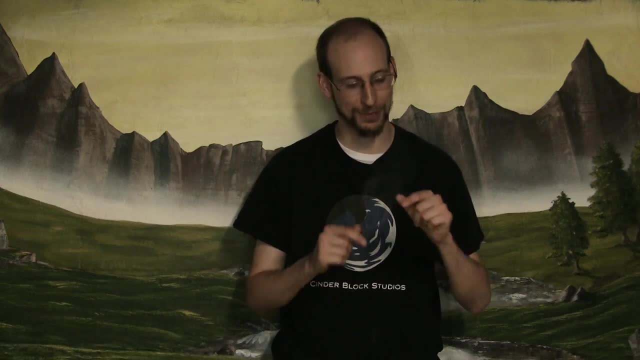 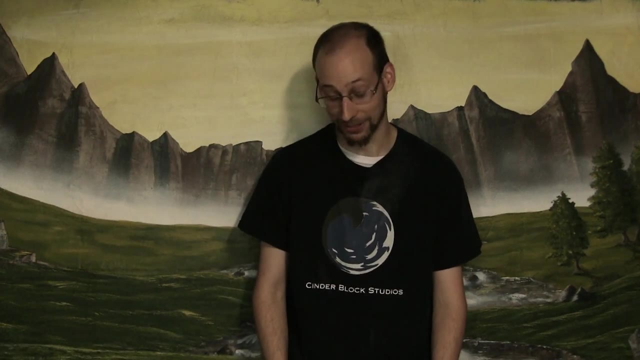 featured in that. So do check that video out as well, And always be sure to subscribe to this channel support on Patreon if you're able to. And this has been Sunderblog Studios and I'll see you guys next time. God. 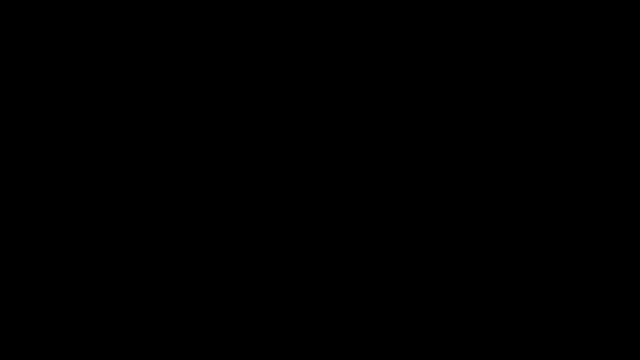 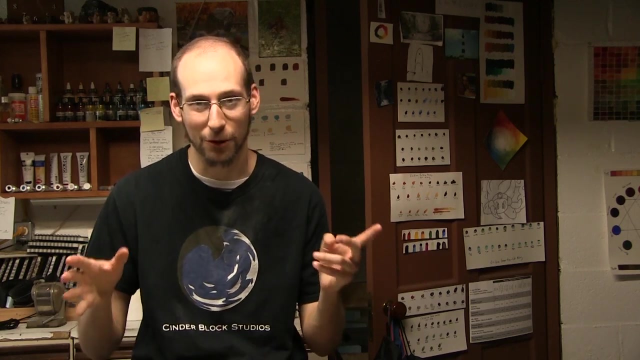 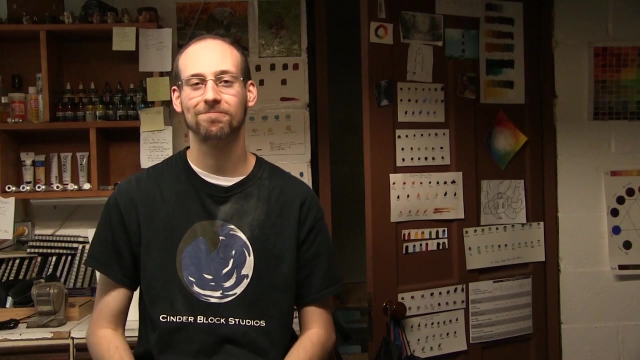 I really flubbed that ending. That's ridiculous And what really any kid is taught when they're younger. The primary colors. when you mix them together, you get a dark Red and blue, make green? No, they don't Wow.